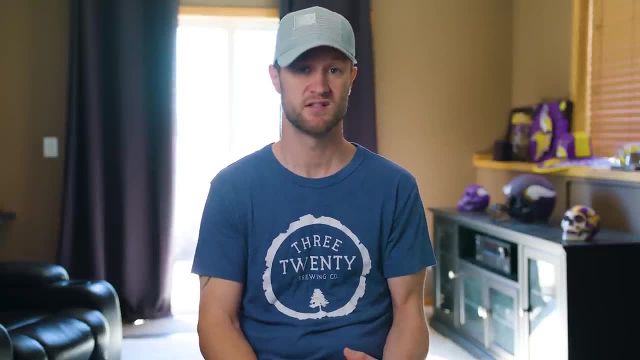 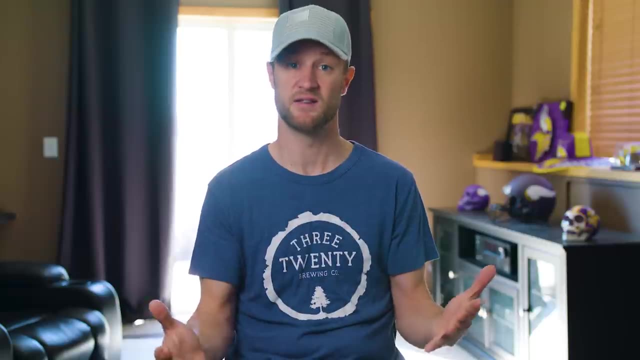 in at once and just kill three birds with one stone. The nitrogen gets your grass dark, The iron really gets your grass dark, and PGR stops the growth of your grass and it gets a dark on top of it. So it's a three dark green cocktail that I like to use. 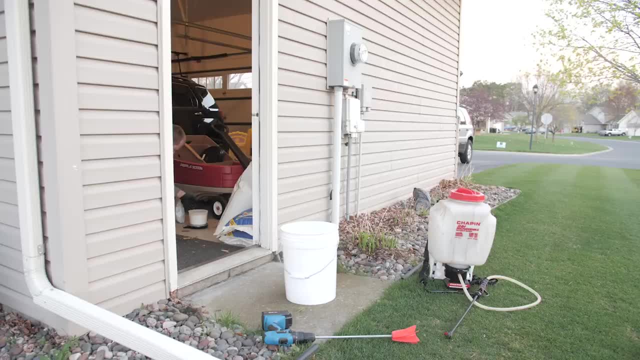 I'm gonna show you guys how to use that cocktail right now. Now, in this bucket I have three and a half gallons of hot water. Now, the reason I use hot water is because it helps everything dissolve a lot easier. I've used cold water when trying to do this process. 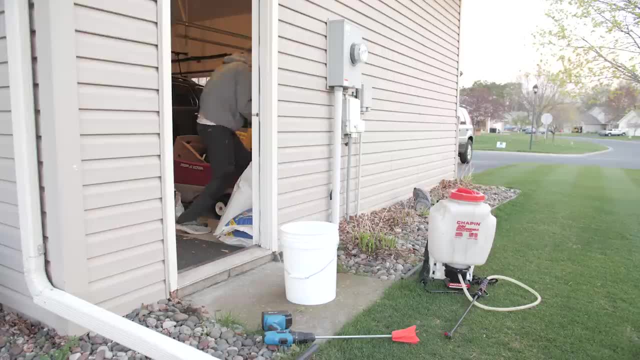 and it just doesn't work very well. It takes a long time for the fertilizer to dissolve and the iron doesn't mix very well in cold water. It just kind of sits at the bottom and just all the sediment just kind of sits there and just goes to the bottom. 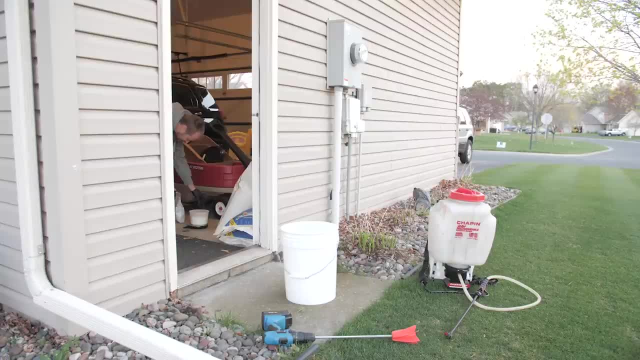 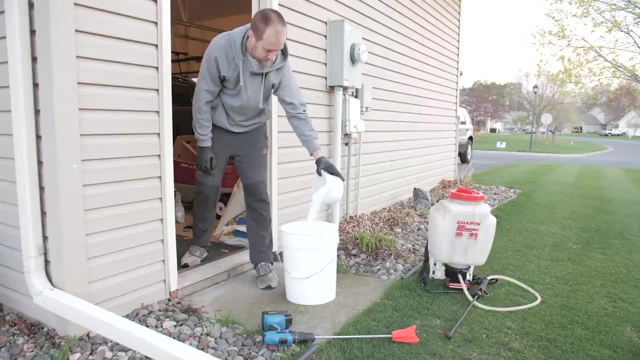 So with hot water it mixes really well. Now I have three and a half gallons of water in this bucket, because I am covering 3,500 square feet, So I am using one gallon of water per thousand square feet. Now, the first ingredient we're adding is nitrogen. 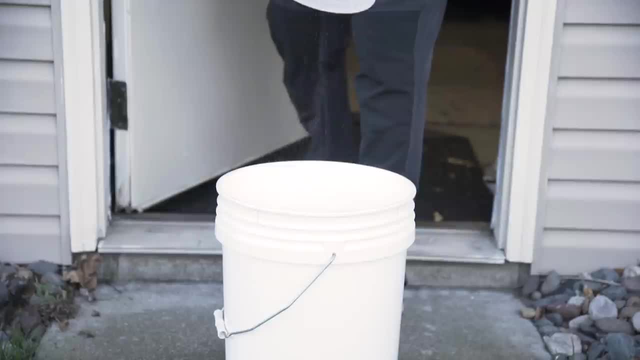 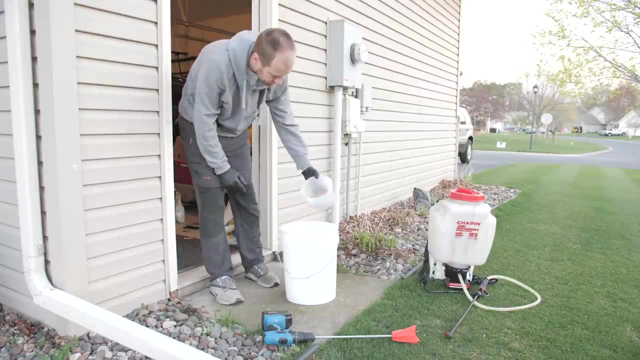 which this is urea. Urea is 46% nitrogen, So I am adding 0.2 pounds of nitrogen per thousand square feet in this cocktail. Now, the second ingredient we're using is iron, and we are using one and a half ounces per thousand. 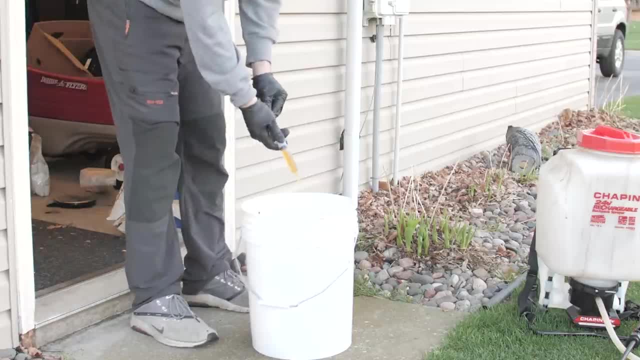 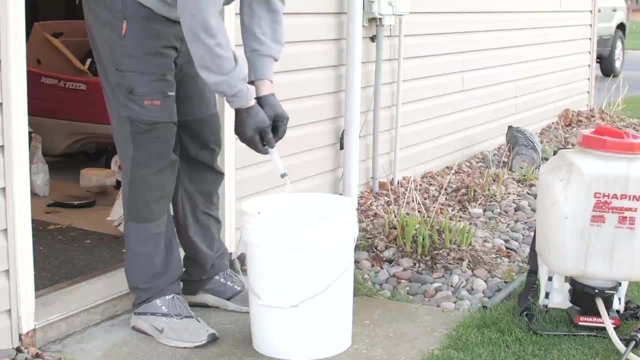 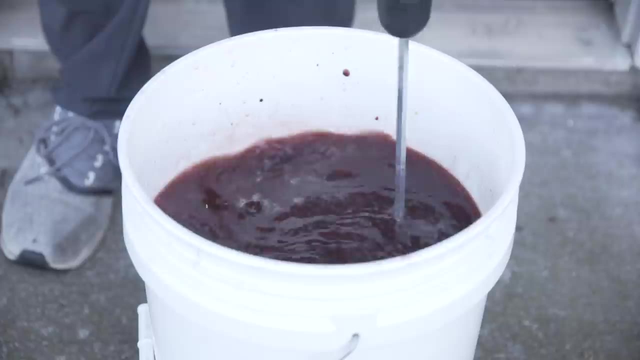 square feet. And the last ingredient is PGR. This is my first application this year, So I'm only putting in five milliliters per thousand square feet. Now go ahead and mix it up as good as you possibly can. Make sure that all of that urea dissolves. 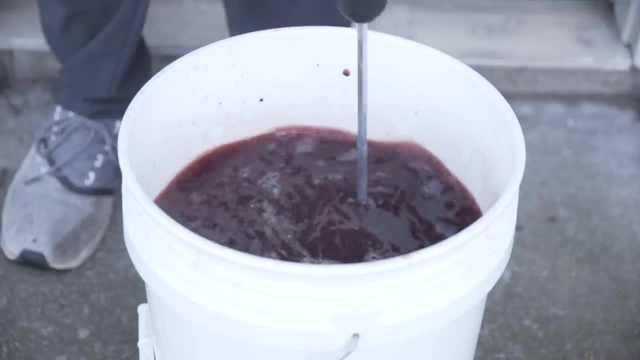 and all the iron is mixed up as good as possible. I would definitely use a strainer when you put this into your backpack, just because there's a lot of sediment and artifacts that could clog up your sprayer. Now I'm leaving this box out here as I spray. 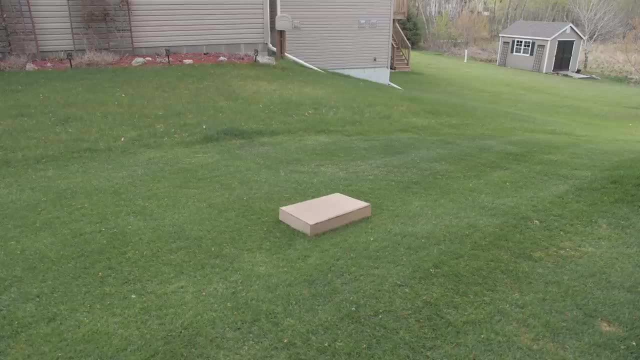 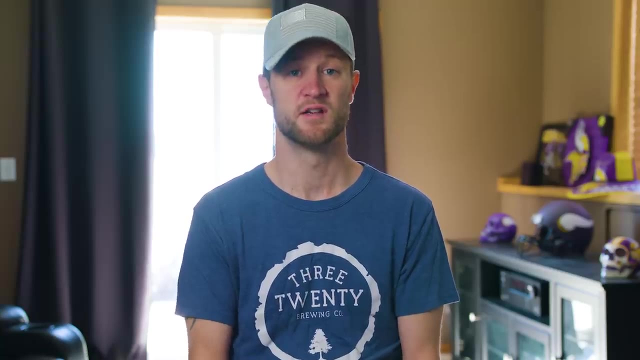 just so we can see what the grass looks like before and after. So that way we'll have a control plot. basically, Now, when it comes to iron, there's not very many negatives that come with it. I mean all the positives that come with iron. 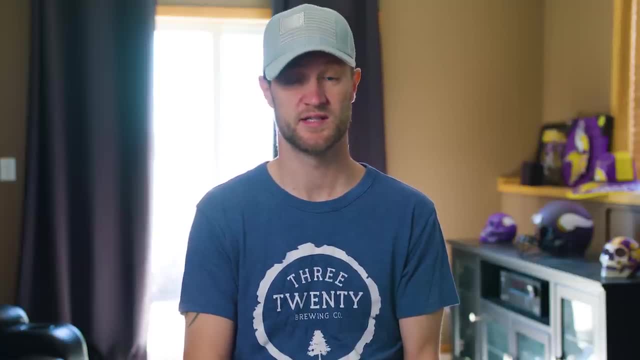 is you get that super dark color. It's super healthy for your grass so it can help fight off disease. It actually needs the nutrient And if you have moss in your soil, if you have moss in your yard for some reason, it actually helps get rid of the moss also. 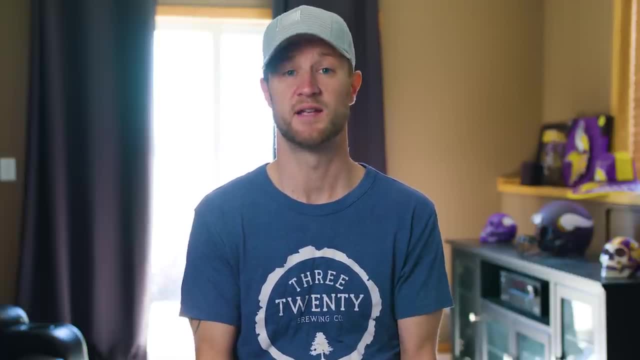 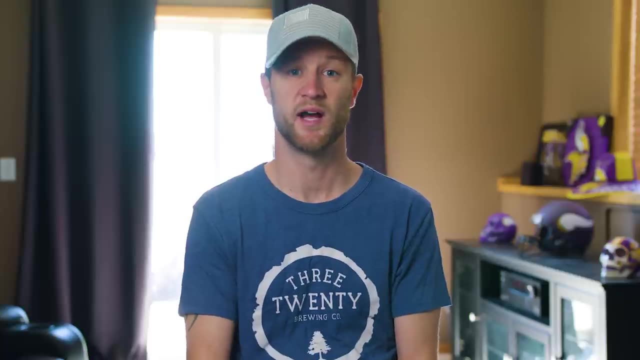 So iron does a ton of things for your grass and it makes it look good at the same time, And it also doesn't make your grass grow any faster, which is awesome, So it doesn't grow super fast after you apply it like nitrogen. 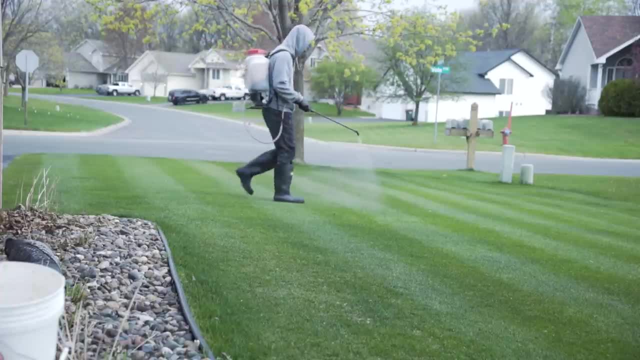 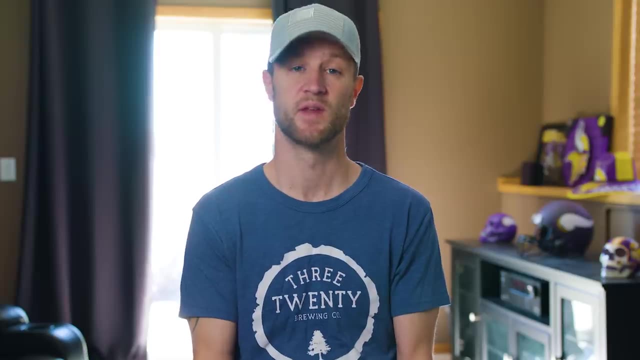 Now, the only drawbacks I really see with iron is that the iron doesn't last that long. When you apply the iron, it only lasts maybe two to three weeks and you have to apply it again to get that same effect. So you have to constantly apply iron to get. 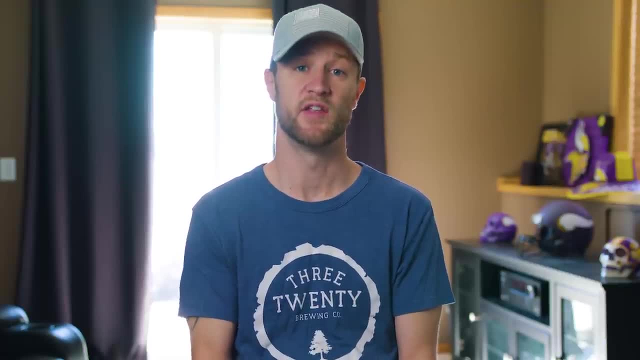 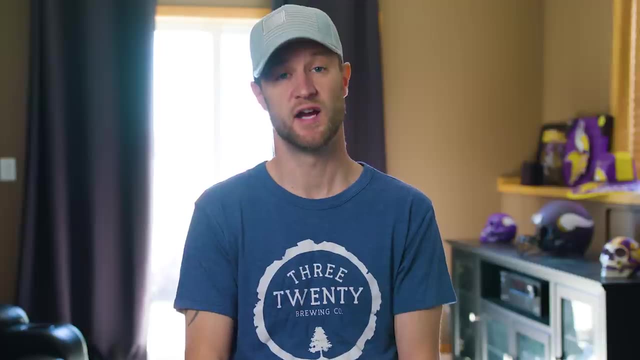 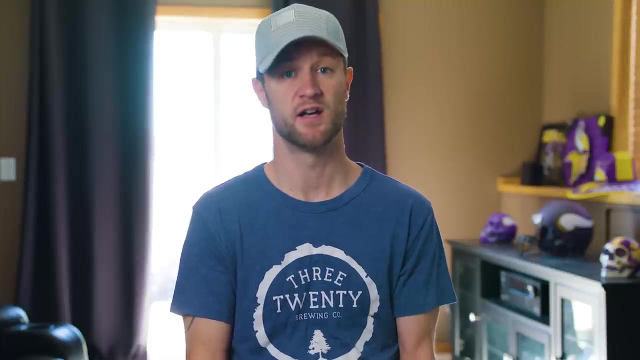 those effects to work. So that would be one negative. The other negative when applying foliar iron is some types of iron can stain concrete. Now, you definitely want to be careful with this. The iron I prefer to use is Feature, which is a chelated iron, and it does not stain concrete. 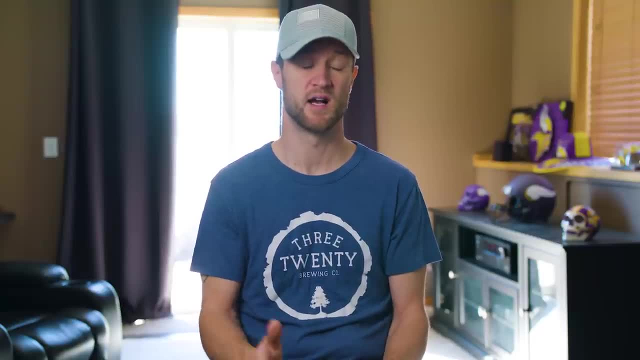 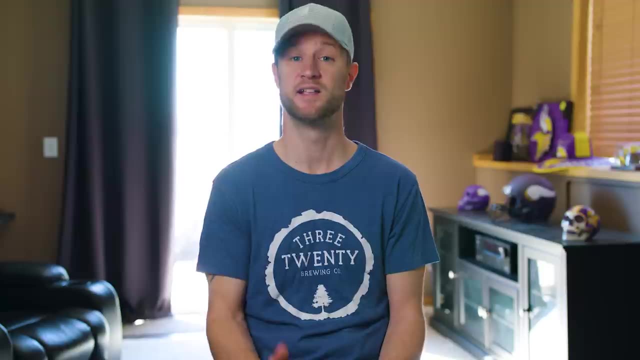 Now, not all chelated irons remove the risk of staining your concrete, So you really got to research whatever product you're going to use and make sure that it doesn't stain your concrete, Because once it stains, it's pretty much there. 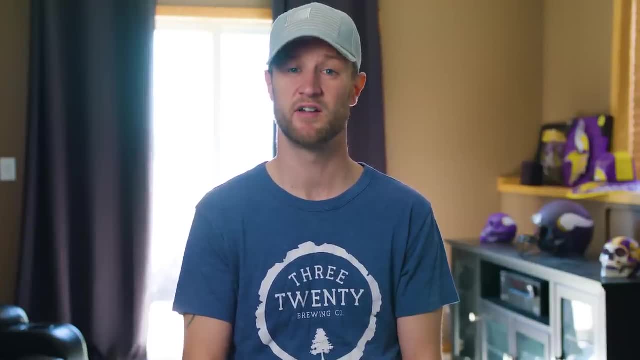 I mean you can. there's a few things you can do to try getting a little bit of it off, But for the most part, once you stain that concrete it's stained orange and it looks bad. So you want to be very careful. 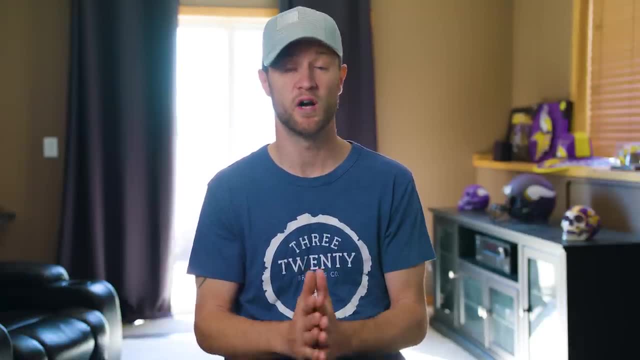 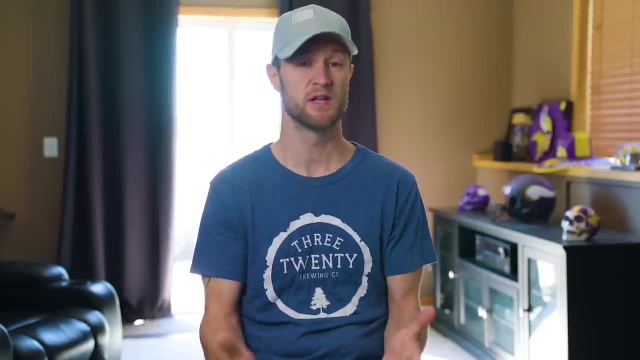 with whatever product you're using Now, be careful not to over apply iron, because your grass will turn black and it looks really weird. So it probably the odds of it killing your grass are very low. Your grass is going to bounce back, but you can definitely over apply iron. 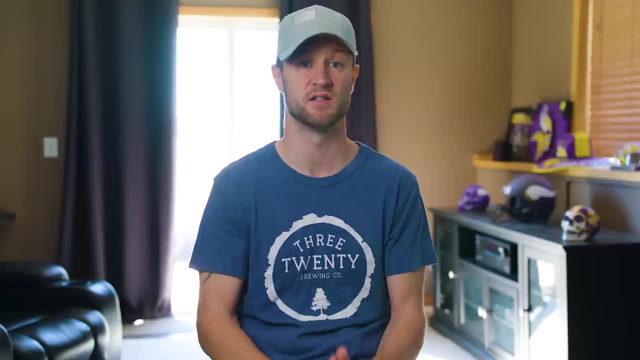 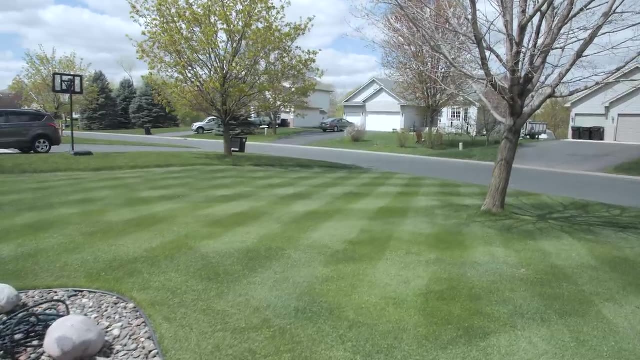 and it's going to look black and then it might turn brown a little bit. It's just going to look super gross. So just be careful that you're not over applying the iron. So here's the grass after I applied that cocktail and after I cut it. 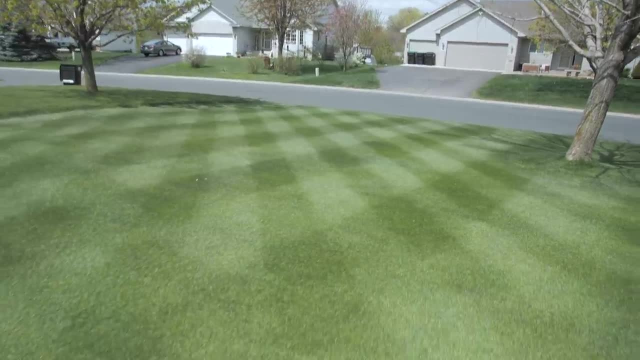 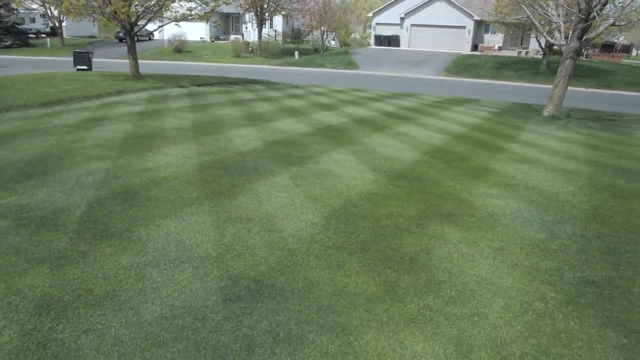 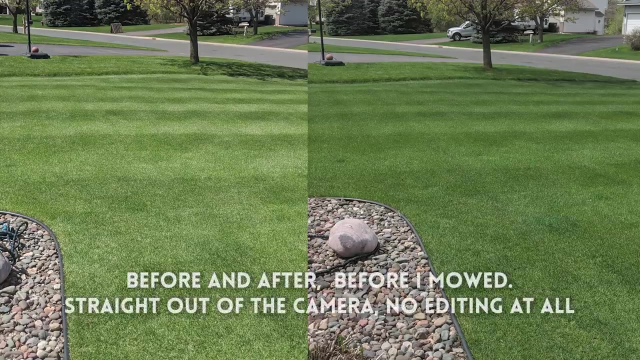 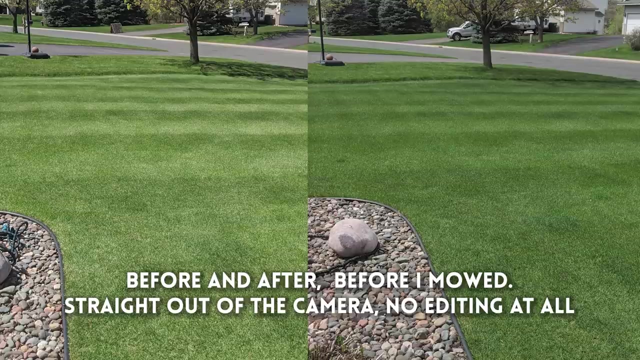 And I'm really kicking myself for cutting the grass, because I should have showed you when it was still a little longer, because it looked way darker than it is right now. I lost a lot of color once I cut it, And that's just the nature of having short grass. 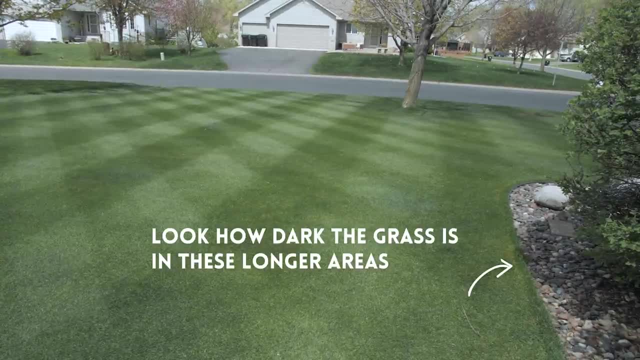 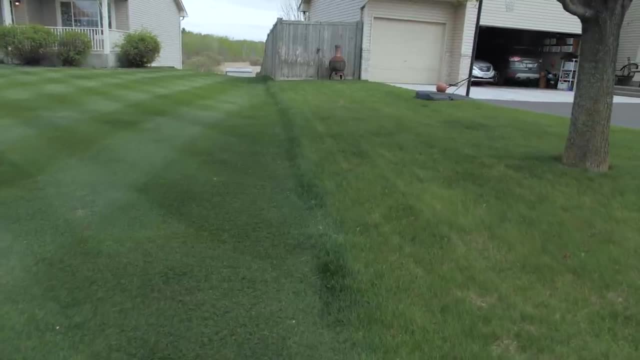 It's hard to really retain color. The shorter you go, the more color you're going to lose. It just is what it is Now. if you look on my neighbor's property line, you can see where I over sprayed and how much darker their grass is. 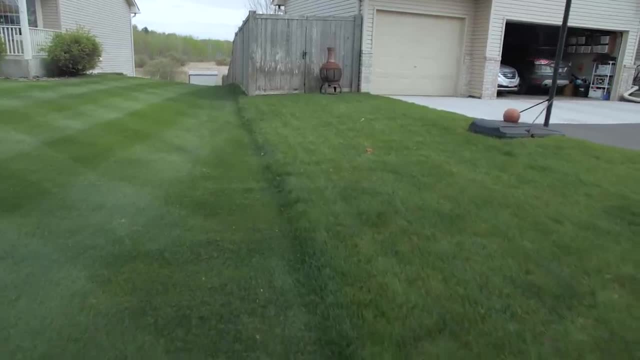 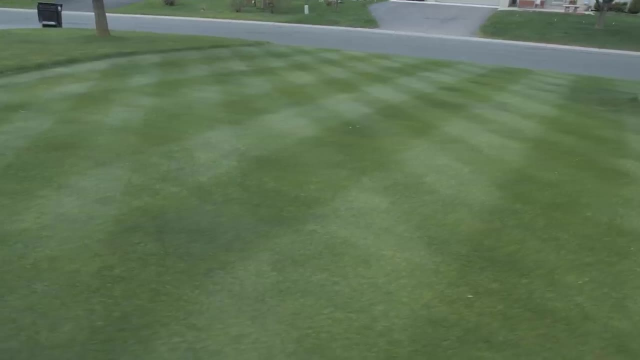 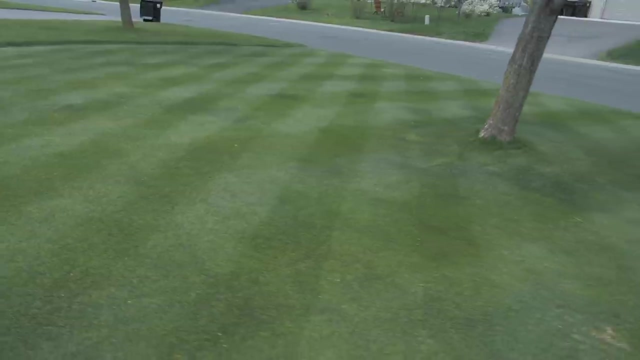 On the spots I hit it, So this would work really well with tall grass. It'd get it super dark, But for how much color I lost? it still looks pretty good. And before people give me crap about how dark my neighbor's grass is across the street, I bet you that stuff's eight to 10 inches in some places. They haven't cut their grass once all year. Just saying, I also did a test area where I covered that box up when I was spraying And you can clearly see where that box was. 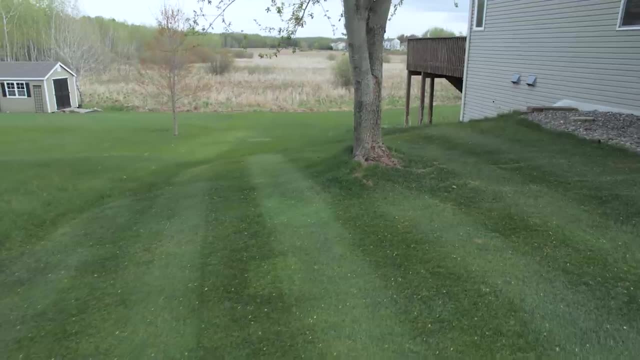 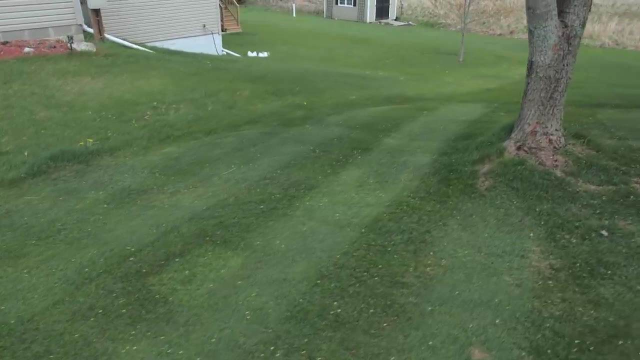 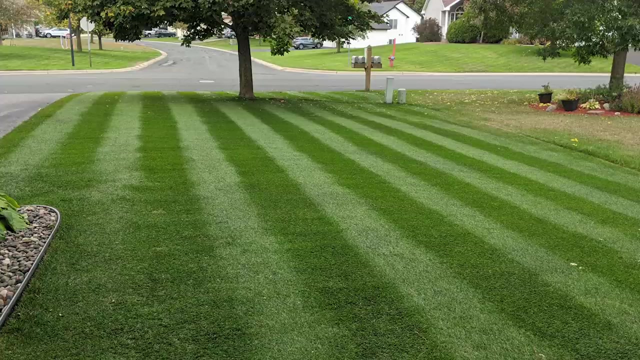 So my grass was a lot lighter before I added that cocktail, So I'm happy how it came out. Last year, after applying this a few times, my grass got super dark, So this is the first time I've applied this this year. 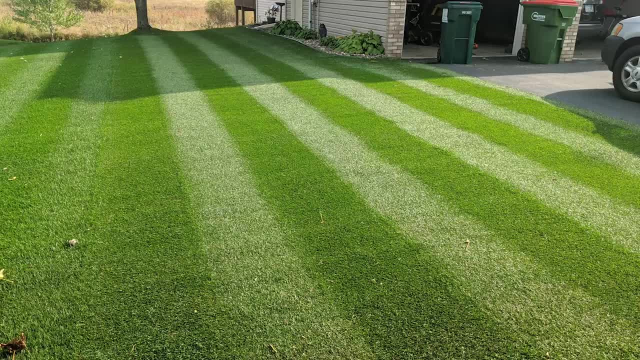 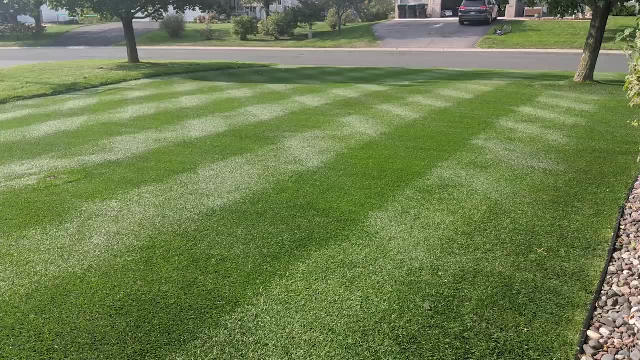 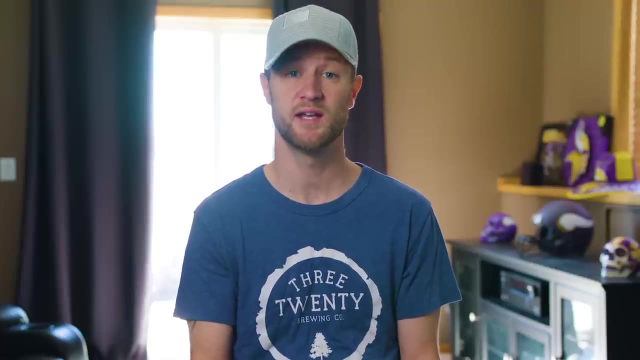 So it's not responding as well as it did last year. after a few apps, I can definitely see the change. So there you have it. There's my three ingredients. This is a convenient cocktail. Like I said, you don't need to put all three in. 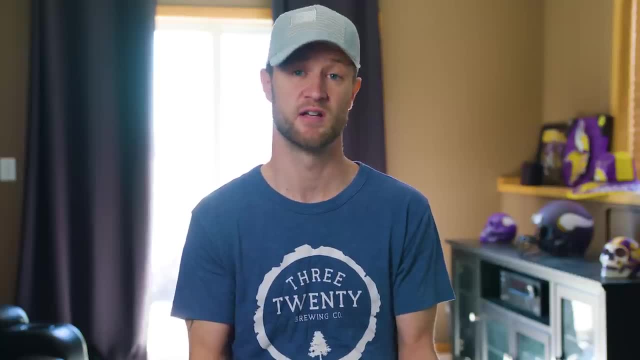 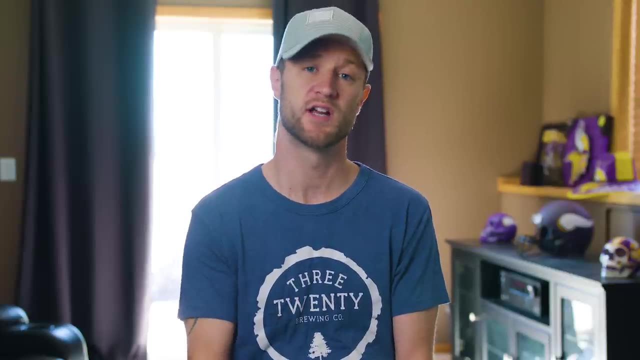 You can just do the iron. It's still gonna get super dark, but I just prefer killing three birds with one stone. If you guys have any questions about foliar applications of iron or iron in general, leave your comments below and I'll be sure to get back to you. 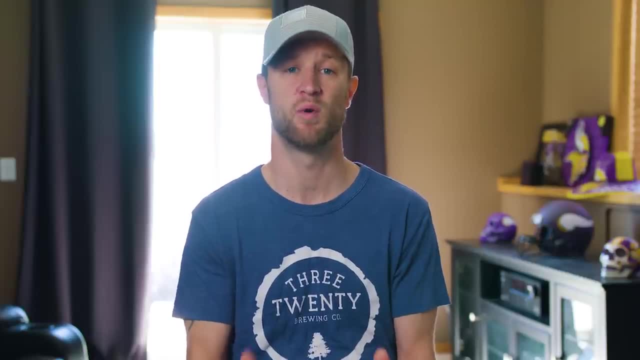 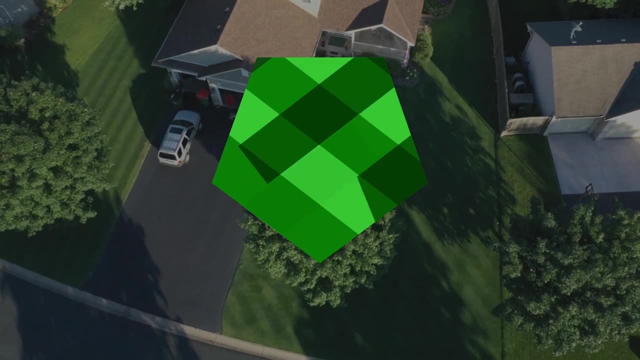 If you guys can subscribe and hit that notification bell, I would really appreciate it. I wanna give you guys as much useful content as possible. Otherwise I'll see you next time on Lawn Life. Bye.